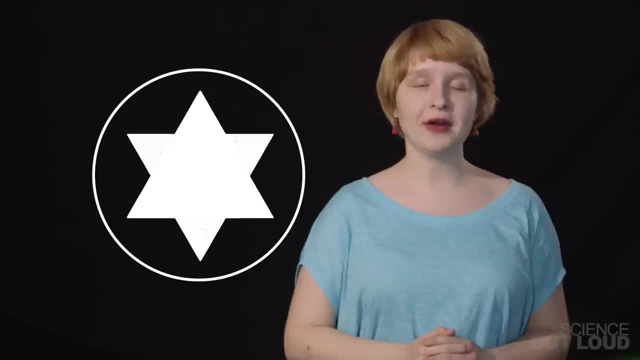 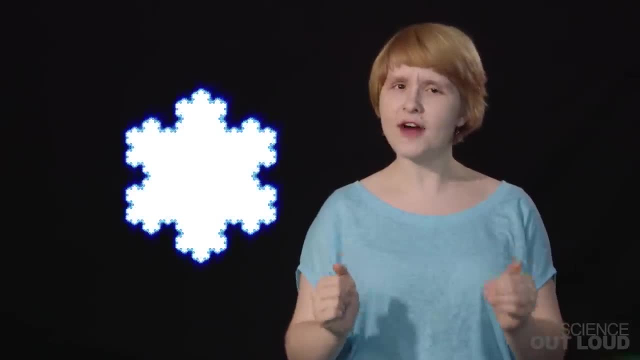 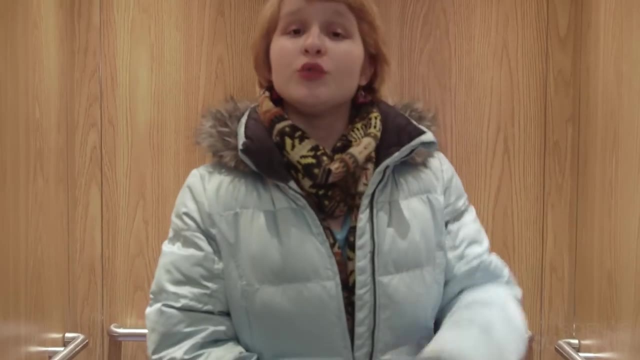 around the snowflake, it will fit completely inside, no matter how many times we increase the number of sides. So the Koch fractal has an infinite perimeter, but a finite area. In the 1990s, a radio astronomer named Nathan Cohen used the fractal antenna to rethink wireless. 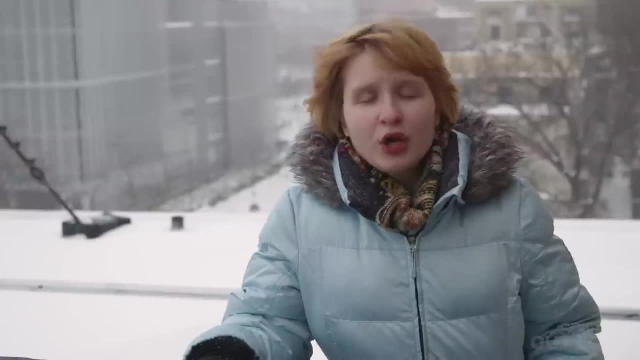 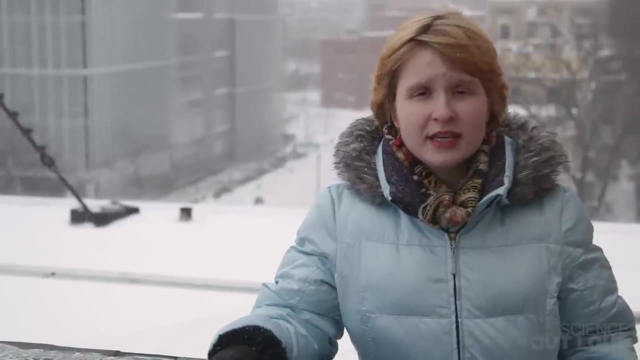 communications At the time. Cohen's landlord wouldn't let him do it. He'd say, well, I don't know what to do with the radio antenna. So he decided to make a more compact fractal-like radio antenna instead. But it didn't just hide the antenna from his landlord, It also 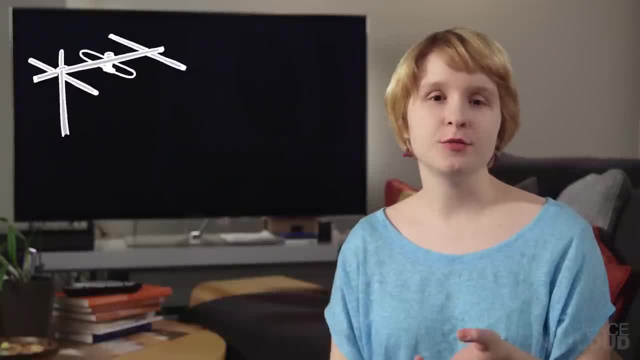 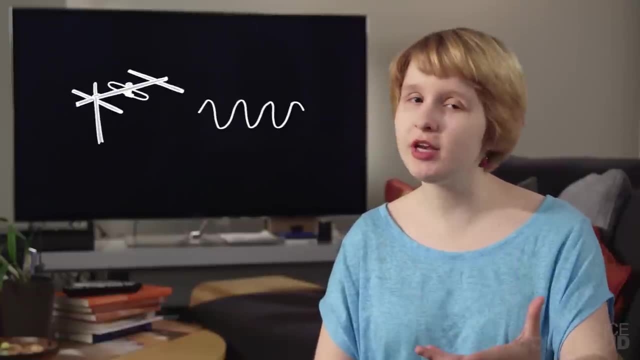 seemed to work better than the regular ones. Regular antennas have to be cut for one type of signal And they usually work best when their lengths are certain multiples of their signal wavelengths. So FM radio antennas can only pick up FM radio stations. TV antennas. 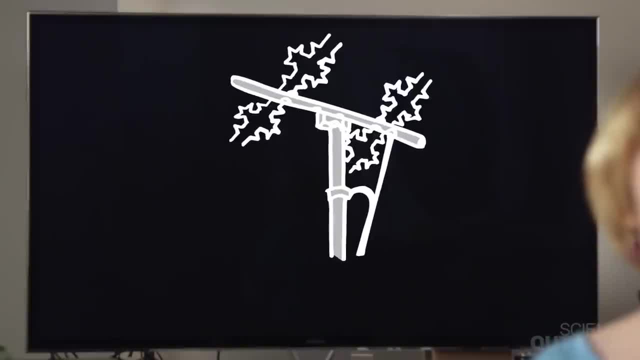 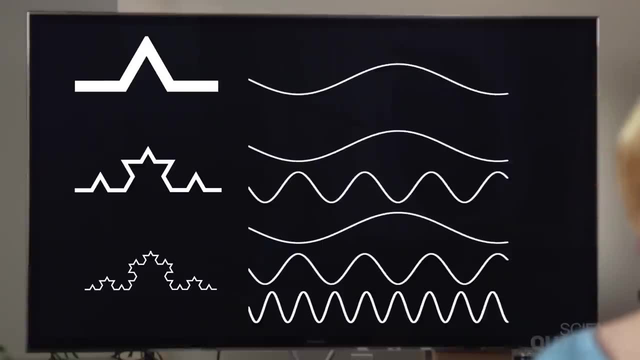 can only pick up TV channels and so on. But fractal antennas are different. As the fractal repeats itself more and more, the fractal antenna can pick up more and more signals, not just one. And because the perimeter of the Koch snowflake grows way faster than its 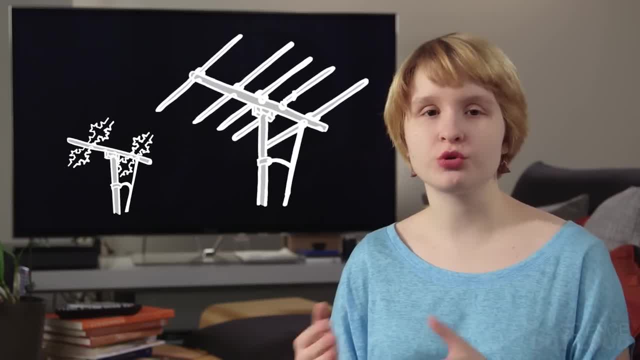 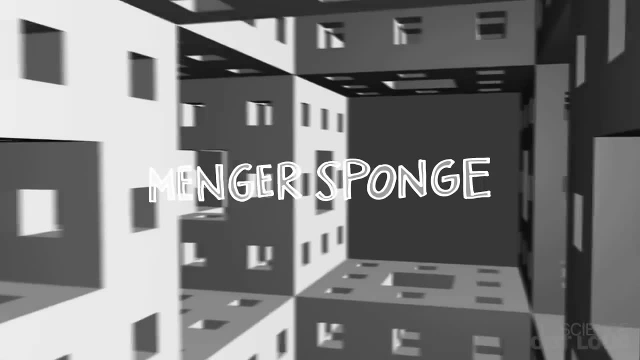 area. the fractal antenna only takes up a quarter of the usual space. But Cohen didn't stop there. He designed a new antenna, this time using a fractal called the Menger sponge. The Menger sponge is kind of like a 3D version of the Koch snowflake: It has infinite surface. area, but finite volume. The Menger sponge is sometimes used in cell phone antennas. It can receive all kinds of signals while taking up even less area than a Koch snowflake. Now, these antennas aren't perfect. They're smaller, but they're also very intricate. 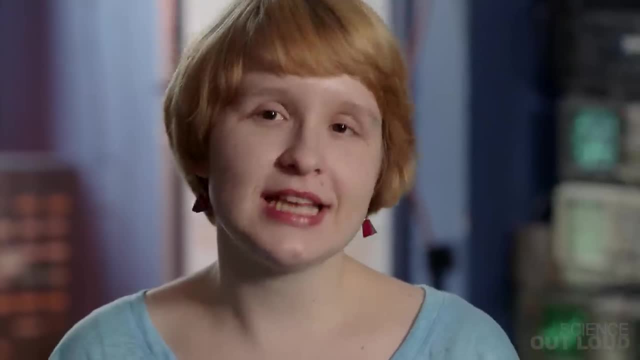 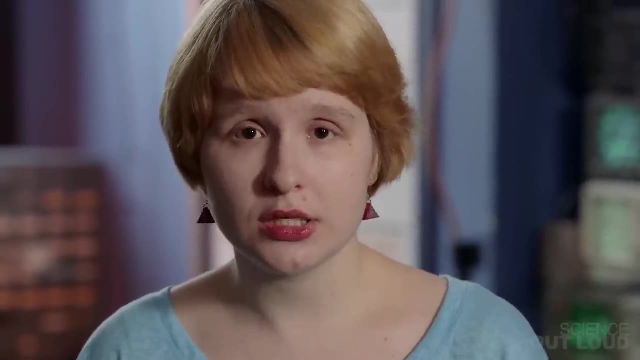 so they're harder and more expensive to make, And although fractal antennas can receive many different types of signals, they can't always receive each signal as well as an antenna that was cut for it. Cohen's invention was not the first application of fractals Nature. 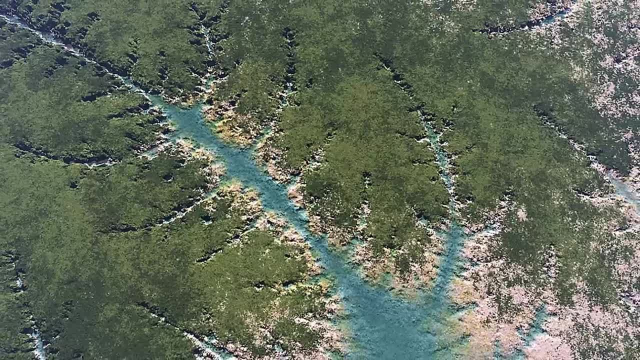 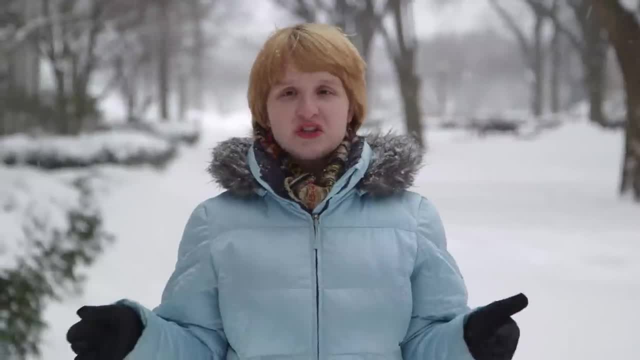 has been doing it forever, and not just with snowflakes. You can see fractals in river systems, lightning bolts, seashells and even whole galaxies. So many natural systems previously thought off-limits to mathematicians can now be explained in terms of fractals.